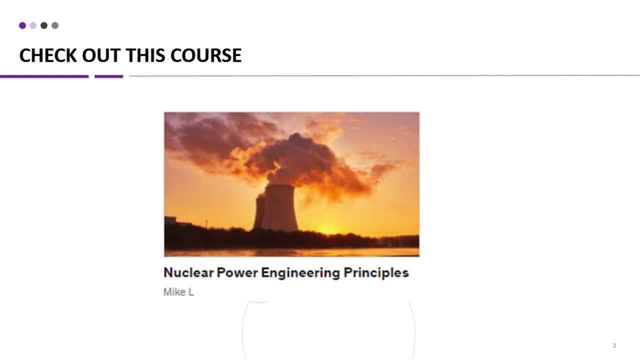 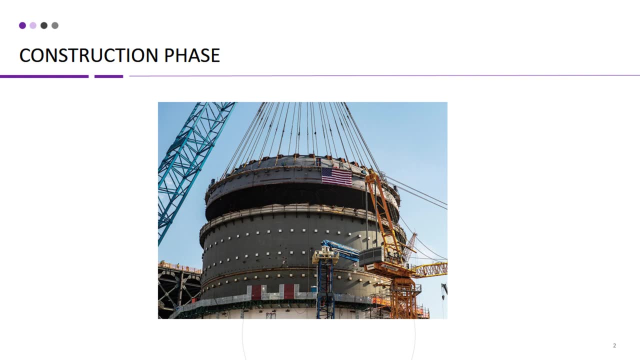 If you're interested, the link to this course is provided in the video description below. The construction phase is the first stage in the life cycle of a nuclear power plant. It involves site selection, obtaining necessary permits and licenses, and building the infrastructure for the plant. Construction of a nuclear power plant is a complex and time-consuming process. 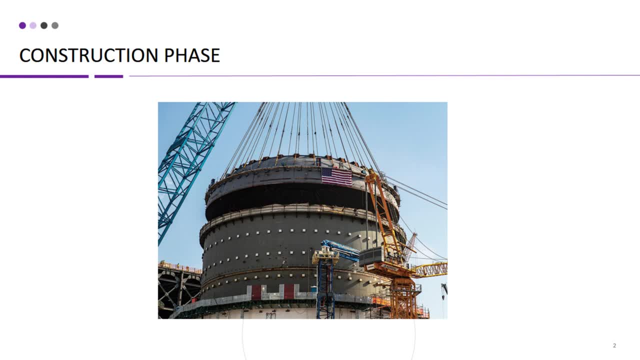 that requires careful planning and adherence to strict safety regulations. The construction phase typically involves several key activities, Including site preparation, excavation, concrete pouring and installation of various components, such as the reactor, turbines and cooling systems. It also involves the installation of safety features. 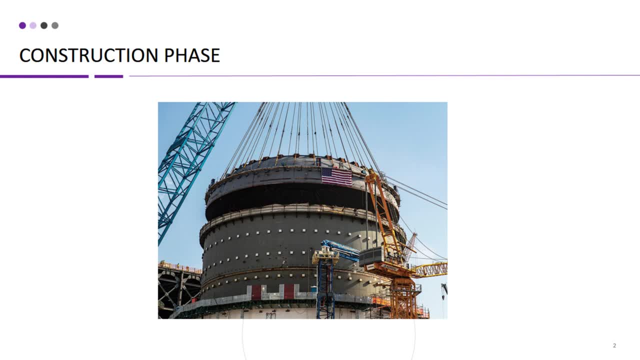 such as containment structures, emergency shutdown systems and radiation protection measures to ensure the safe operation of the plant. Safety is a top priority in every phase of a nuclear power plant's life. Nuclear Power Engineering Principles is a top priority in every phase of a nuclear power plant's life. 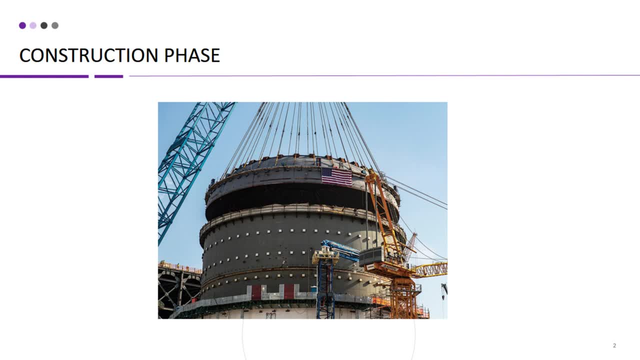 Nuclear Power Engineering Principles is a top priority in every phase of a nuclear power plant's life. Nuclear Power Engineering Principles is a top priority in every phase of a nuclear power plant's life. The construction phase can take several years or even decades, depending on the size and complexity of the plant. 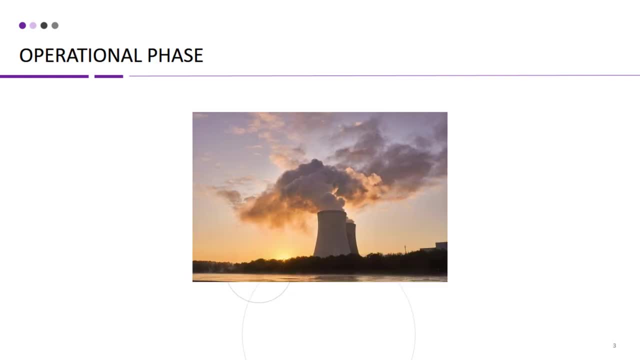 Once construction is complete, the nuclear power plant enters the operational phase where it generates electricity by harnessing the energy from nuclear fission reactions. During this phase, the plant is subject to rigorous safety protocols, regulations and inspections to ensure safe and efficient operation of the plant. 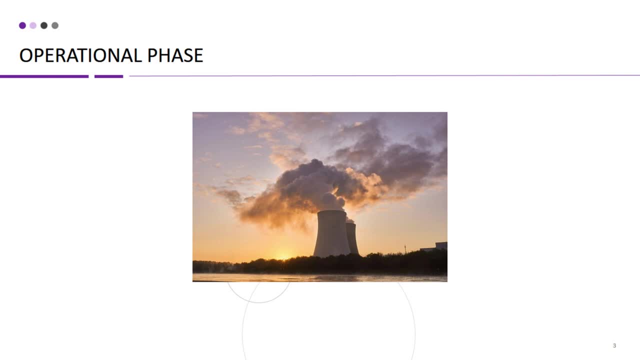 Nuclear Power Engineering Principles is a top priority in every phase of a nuclear power plant's life and efficient operation. The operational phase involves the regular operation of the plant, including the loading of nuclear fuel into the reactor, the controlled fission reactions that generate heat and the production of electricity through a steam turbine. The plant also requires 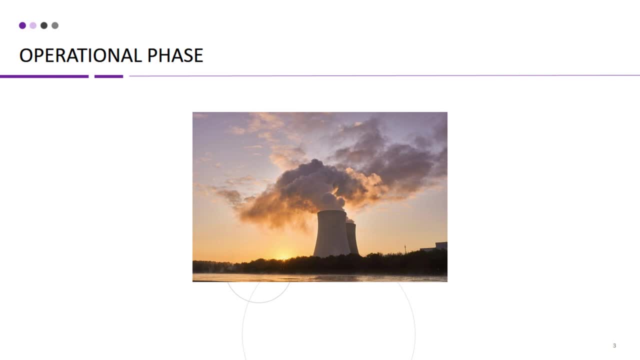 ongoing maintenance, inspections and upgrades to ensure its safe and reliable operation. Additionally, the operational phase involves the management of nuclear waste generated during the power generation process. Nuclear power plants generate spent fuel, which is highly radioactive and requires careful handling, storage and disposal according to regulatory guidelines. 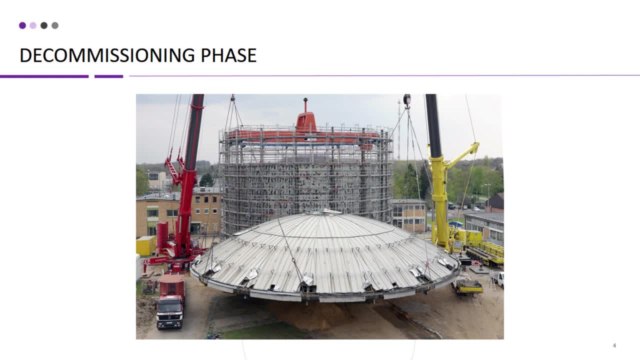 After the operational phase, a nuclear power plant eventually reaches the end of its useful life and enters the decommissioning phase. Decommissioning involves the safe removal of the plant from service and managing its components and radioactive materials in a responsible manner. Decommissioning can be a complex and lengthy 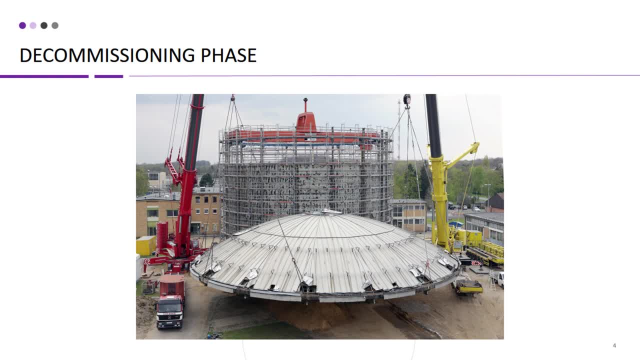 process that includes decontamination, dismantling of structures and waste management. There are different decommissioning strategies, including immediate dismantling, deferred dismantling and entombment, depending on regulatory requirements, safety considerations and the quality of the plant. The decommissioning process is a complex and lengthy process that includes 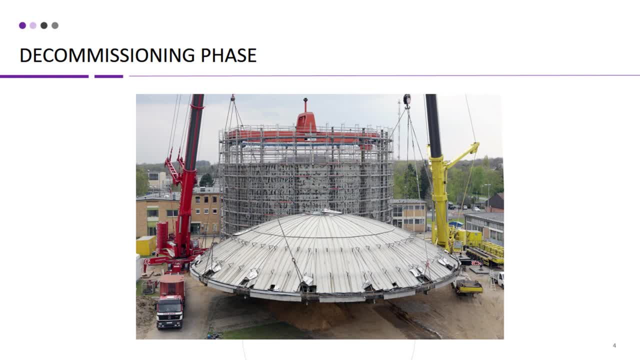 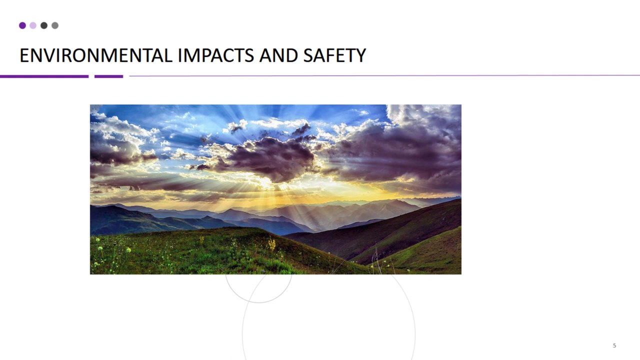 the removal and treatment of radioactive materials, dismantling of buildings and equipment, and site restoration. The goal is to ensure that the site is safely and responsibly managed and any potential risks to human health and the environment are mitigated Throughout the life cycle of a nuclear 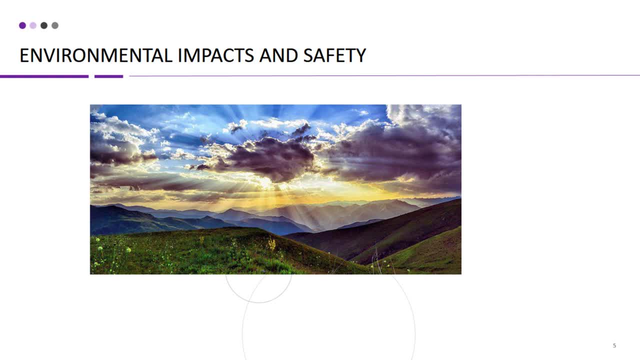 power plant. there are potential environmental impacts and safety considerations that the plant needs to be addressed During the construction phase. potential impacts may include habitat destruction, soil erosion and water pollution. The operational phase requires strict safety protocols and measures to prevent accidents, releases of radioactive materials and protect. 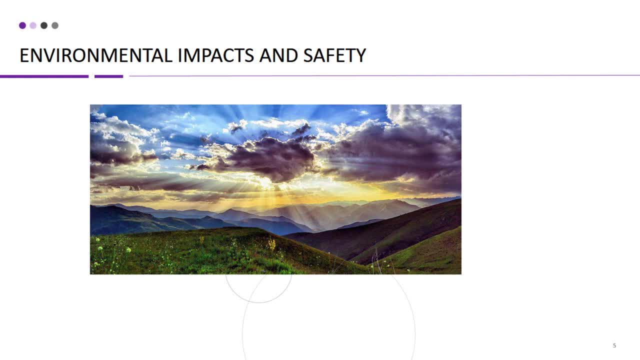 workers and the public. Proper management of nuclear waste, including spent fuel, is crucial to avoid potential environmental and health risks During the decommissioning phase. careful handling of radioactive materials, waste disposal and site restoration are essential to minimize potential impacts on the environment and. 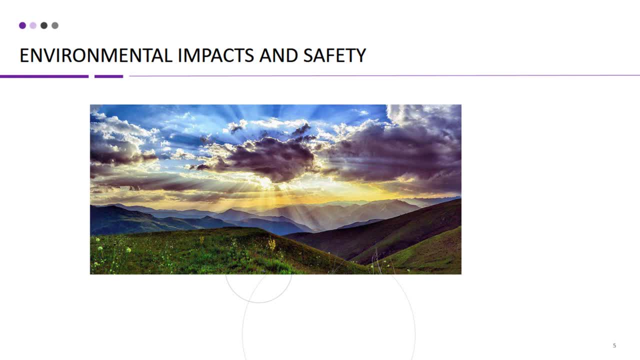 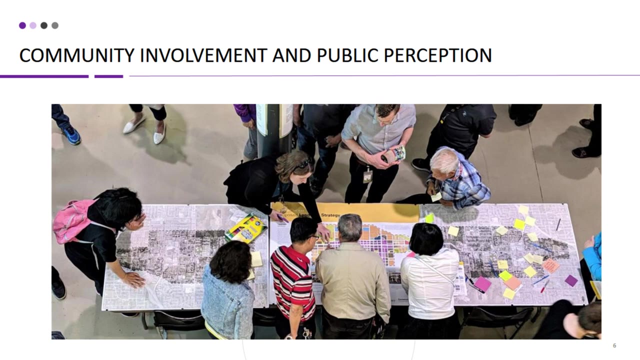 surrounding communities. Safety measures, regulations and oversight by regulatory bodies play a vital role in ensuring the safe operation and decommissioning of nuclear power plants. Another important aspect of the life cycle of a nuclear power plant is community involvement and public perception. Nuclear power plants are often subject to public scrutiny and concerns about safety. 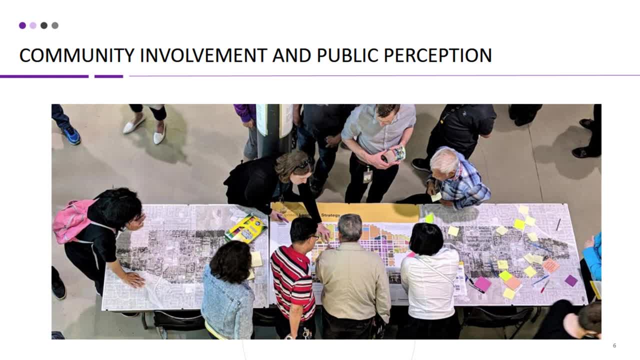 environmental impacts and the handling of radioactive materials. It's crucial for nuclear power plant operators to engage with local communities, address their concerns and provide transparent information about the safety measures, regulations and environmental impacts associated with the plant's operation and decommissioning. 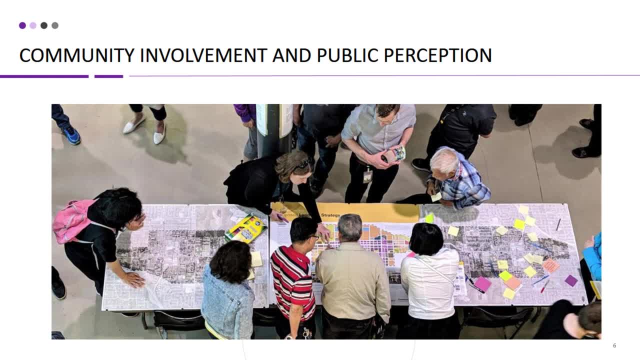 Community involvement and public perception can also play a role in the decision-making process for site selection, construction and decommissioning of nuclear power plants. Building trust and maintaining open communication with the public are essential to ensure a positive perception of nuclear power as a viable energy source. 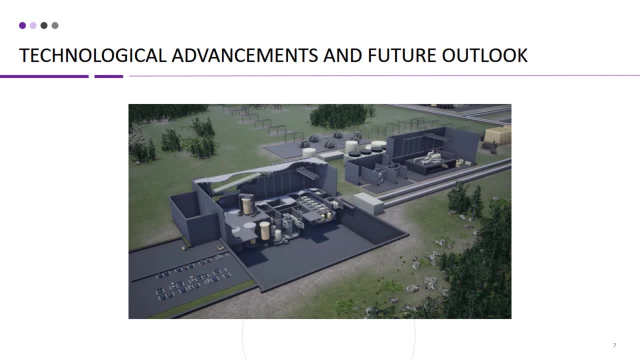 As technology continues to evolve, there are potential advancements that could impact the life cycle of nuclear power plants. Advanced reactor designs, improved safety features and more efficient waste management techniques are being researched and developed to further enhance the safety and sustainability of nuclear power. 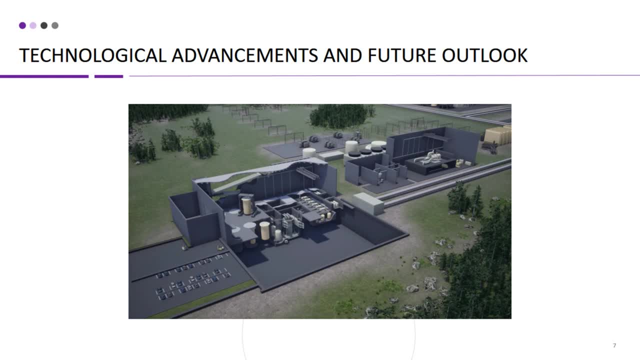 Advanced reactors such as small modular reactors and Generation IV reactors offer potential benefits in terms of safety, efficiency and waste reduction. These advancements could impact the construction of nuclear power plants. In addition, the future outlook for nuclear power will depend on various factors, including regulatory frameworks, public perception, energy demand and technological advancements. 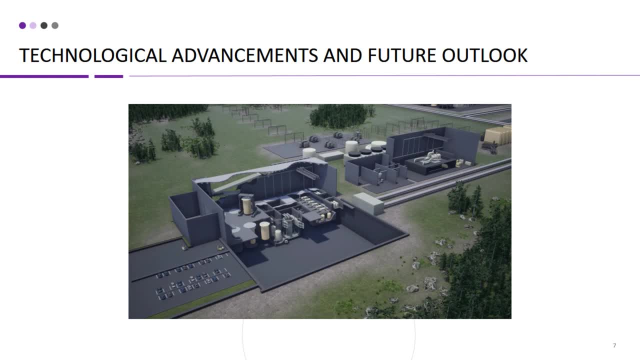 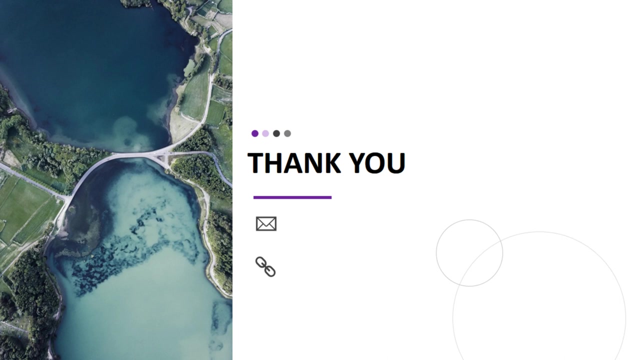 As the world continues to seek low-carbon energy sources to mitigate climate change, nuclear power could play a significant role in the future. Thank you for watching And ensure you become a part of the community of professionals and people invested in all, let us notıyla. 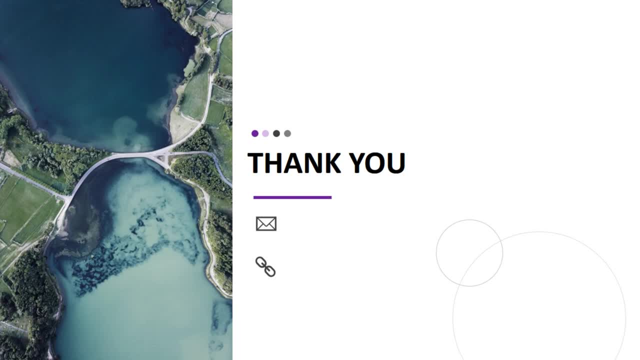 And that brings us to the end of our video on the life cycle of a nuclear power plant. from construction to decommissioning, A power plant is a complex and carefully regulated process that involves safety measures, environmental considerations and community engagement to ensure responsible and sustainable operation.